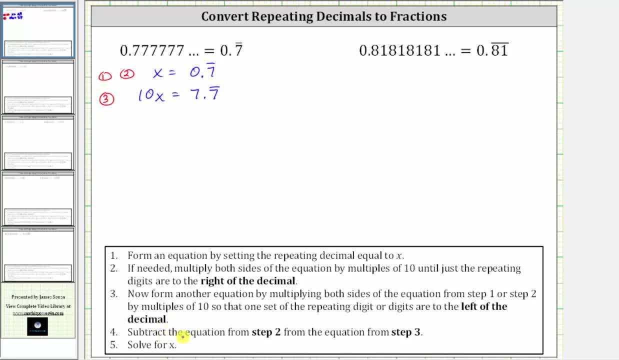 Let's label this equation. This is equation three. And now step four. we subtract the equation from step two from the equation from step three. So, beginning with equation three, we have 10x equals 7.7, repeating. And now I subtract equation two. 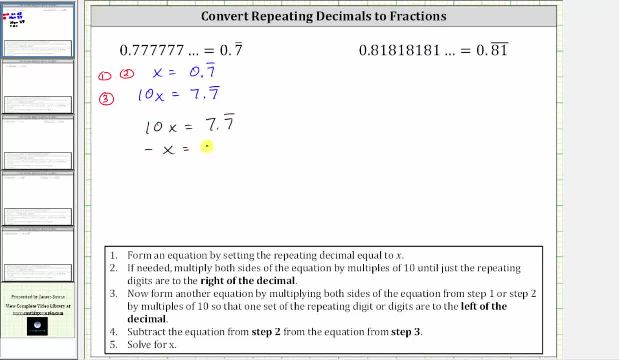 which means we subtract x from the left and we subtract 0.7 repeating from the right. And now subtracting 10x minus x or 10x minus 1x is 9x. Equals, on the right, 7.7 repeating. 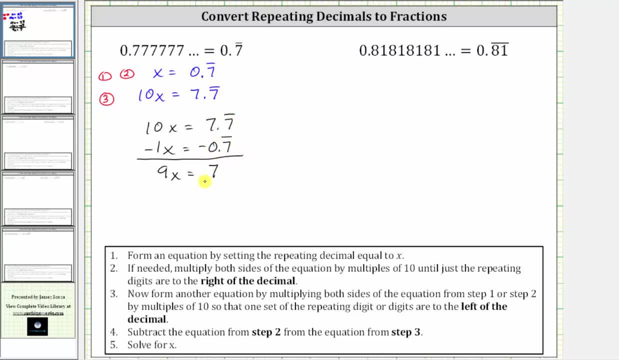 minus 0.7 repeating is equal to seven. And now we solve for x by dividing both sides by nine. Simplifying nine divided by nine is equal to one. One times x is x. We have: x equals 7 ninths. 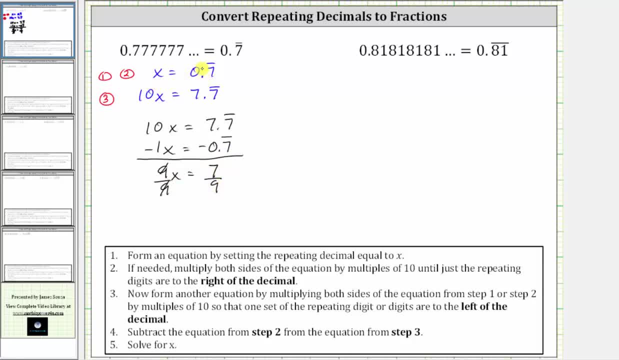 which does not simplify. And since x is equal to the repeating decimal, we now know that 0.7 repeating is equal to the fraction of 7 ninths. So the next example: we begin by setting x equal to 0.81 repeating. 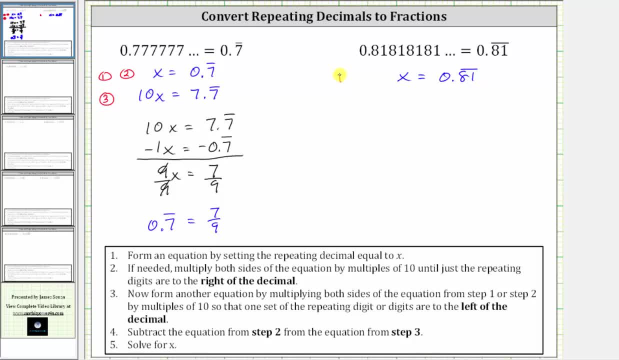 This is from step one. Let's label this equation one. Step two, if needed again, we multiply both sides of the equation by multiples of 10 until just the repeating digits are to the right of the decimal, And for this example, just the eight and one repeating. 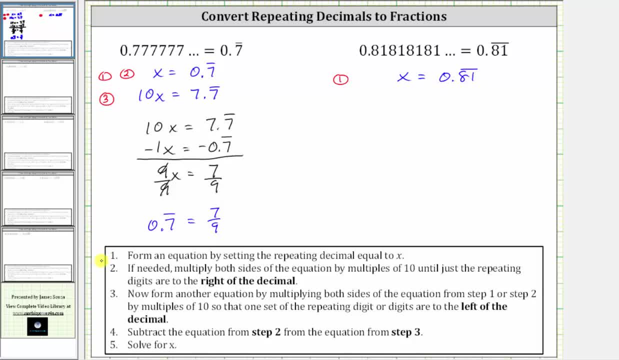 are to the right of the decimal And therefore the condition from step two is already met by this equation. So let's also label this equation two. This won't always be the case, which we will see in future examples. Step three: we now form another equation. 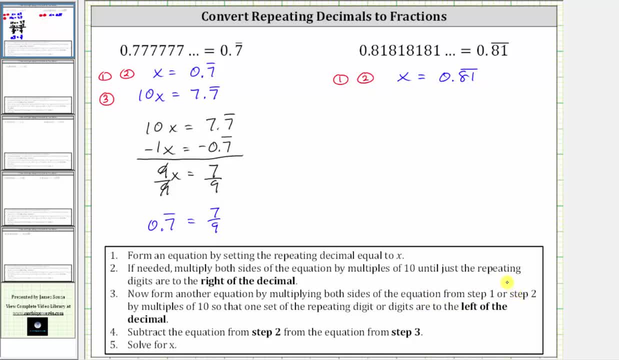 by multiplying both sides of the equation from step one or step two by multiples of 10, so that one set of the repeating digit or digits are now to the left of the decimal, Because the eight and one both repeat. we now need another equation where we have an eight and one to the left of the decimal. 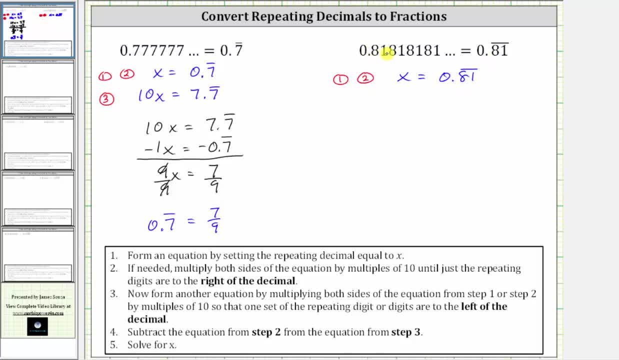 To do this, notice how- here this is the decimal- how we would have to move the decimal two places to the right, which is equivalent to multiplying by 100.. So now we take this equation and multiply both sides by 100.. So for equation 3, we have 100 times x, which is 100x equals 100.